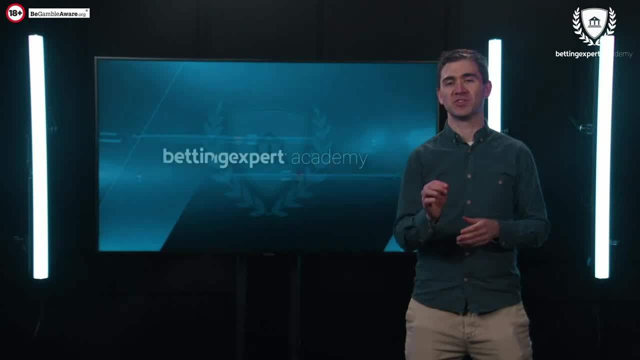 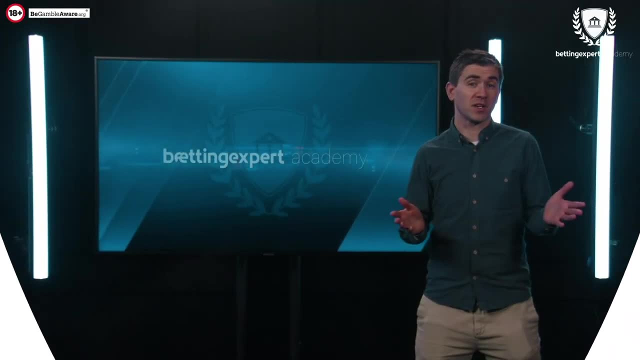 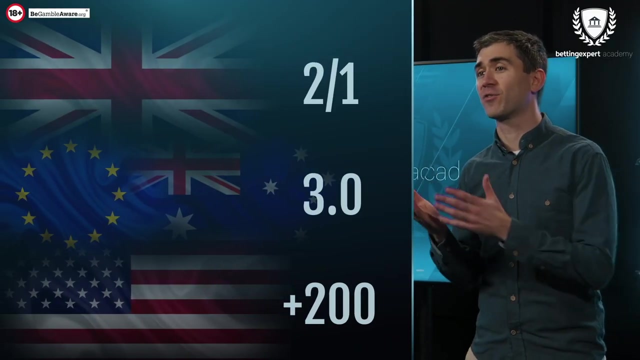 betting odds and convert them to an easy to understand percentage number. So, to start off with, when you look at a betting market on a bookmaker site, you'll see betting odds in one of three different formats: Fractional, which is mostly used in the UK. Decimal, which is popular around Europe or Australia. 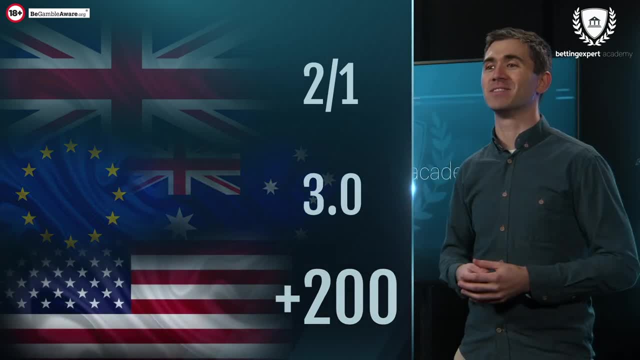 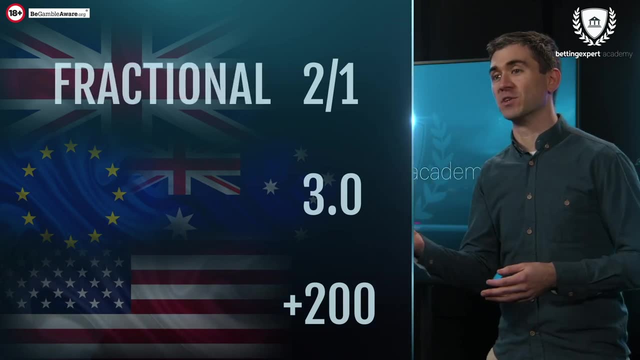 And American odds, which you can probably guess is mainly used in the United States. Fractional odds show you an amount that you could win and the amount you need to stake to win that first amount. Decimal odds show you what your total return would be for a single unit stake. 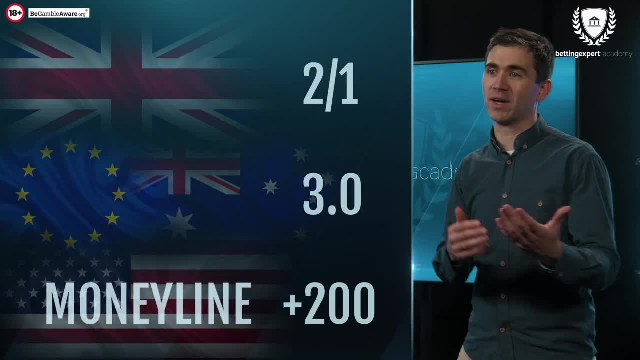 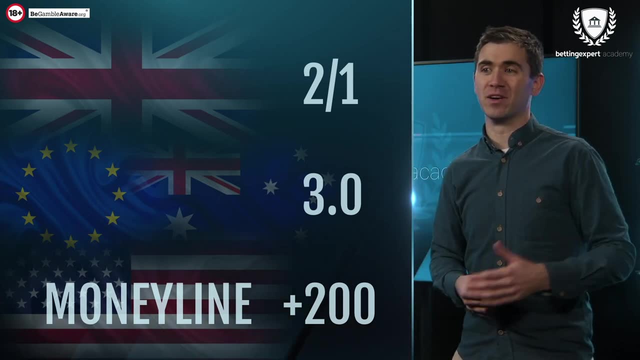 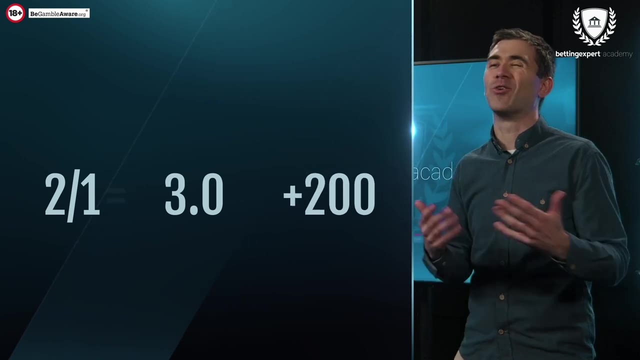 And American odds, which will be shown on either plus or minus, shows either the amount you can win if you stake $100, that's the plus odds- or the amount you need to stake to win $100, that is when the odds are minus. So you could see 2 to 1,, 3.0 or plus 200, and they all mean 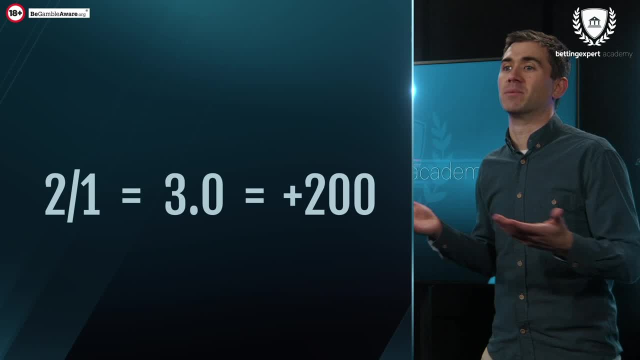 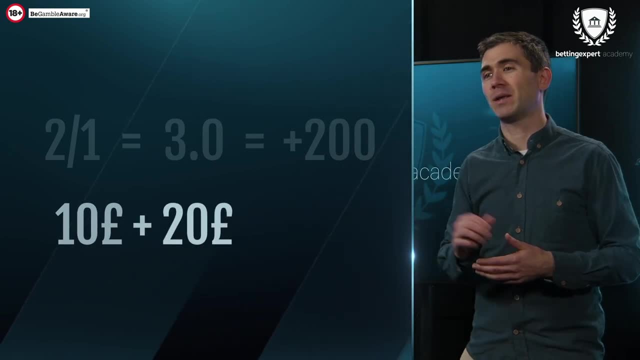 the same thing: Stake a certain amount and you'll get a certain amount back if your bet wins. In this case, if I bet £10 at 2 to 1,, 3.0 or plus 200, I'd win £20 profit and get my stake back. 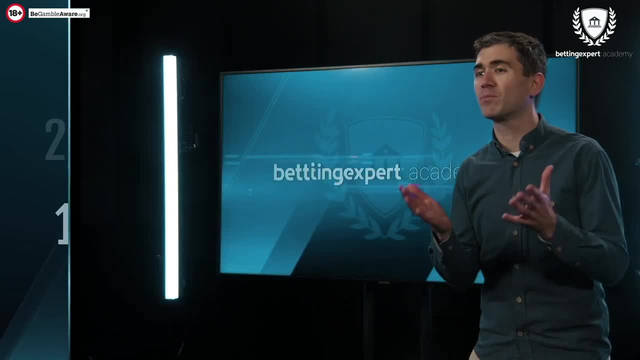 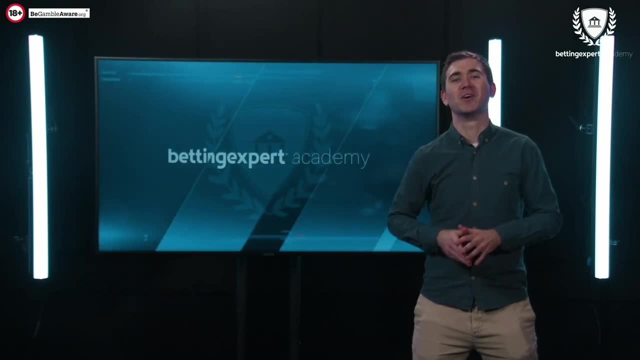 giving a return of £30.. What is the implied probability of winning? Well, this is where we're going to get some formulas out, but don't worry, it's not that scary once you know how it all works. So, starting off with fractional odds Now, if you remember back from your maths lessons at school, 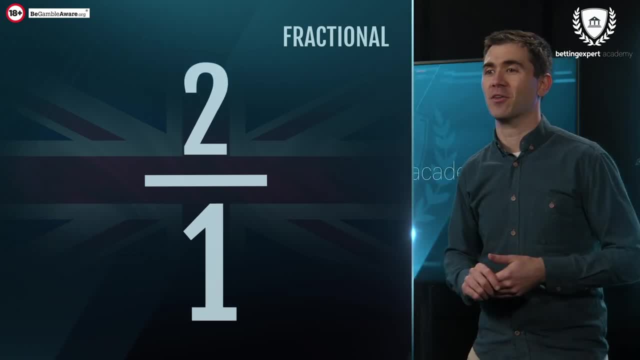 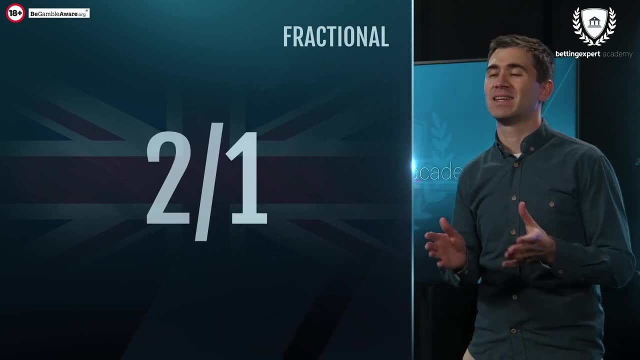 a fraction is made of a numerator on top and a denominator on the bottom. So for our 2 to 1 example, 2 is the numerator and 1 is the denominator. Now the formula to use here is to take the denominator and divide it by the numerator. 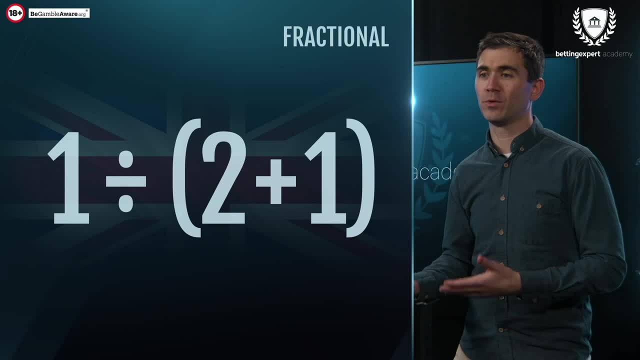 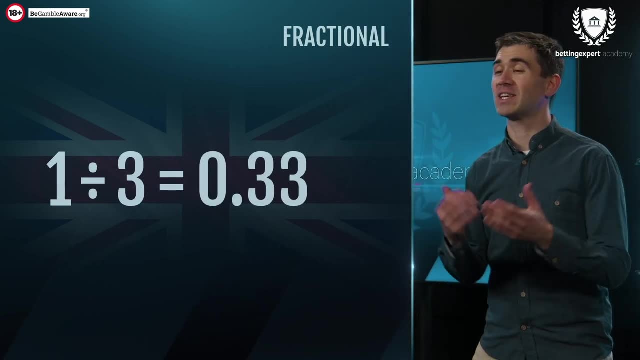 and denominator added together. For our 2 to 1 example, that means 1, divided by 2 plus 1, or 1 divided by 3,, giving 0.33 recurring, which, if you then multiply by 100,. 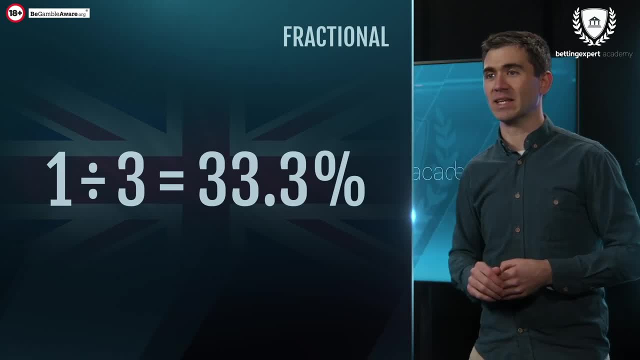 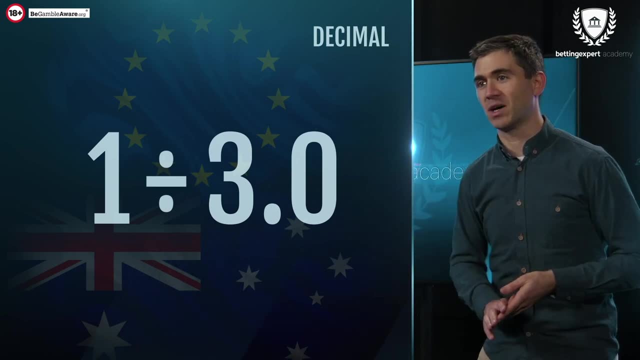 you get 33.3% implied probability. Now for decimal odds. the calculation is 1 divided by those decimal odds. So again, if we take the 3.0 example, we get 1 divided by 3, giving 33.3%. 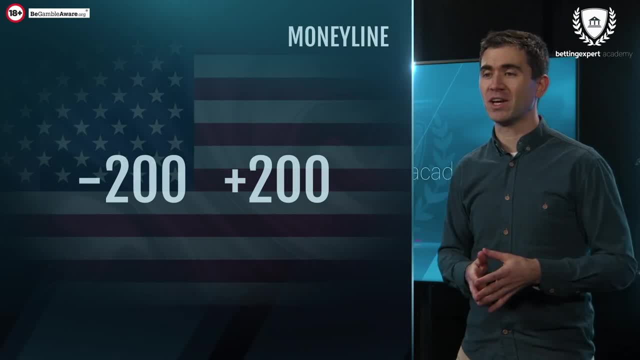 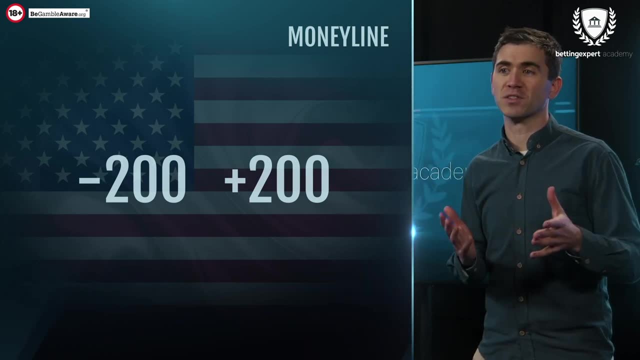 Now for American odds. as I said before, there are two possible variations, plus and minus, and it takes two different formulas to calculate the implied probability depending on which version the odds are. For. plus American odds, you take 100 and divide it by the odds plus 100. 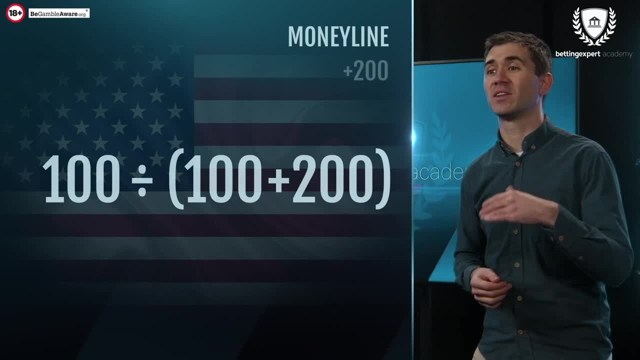 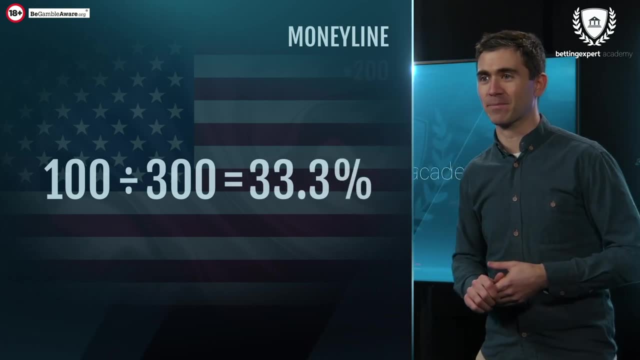 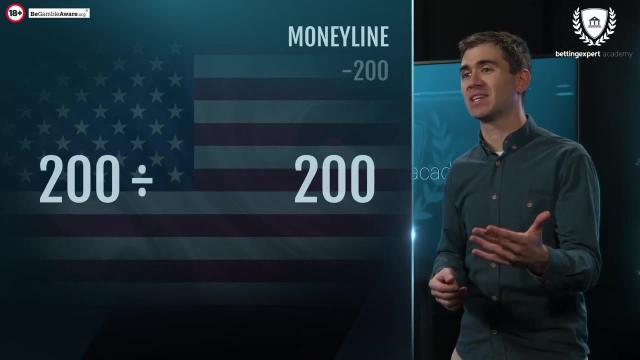 So for our plus 200 example from before, it's 100 divided by 300, which once again gives 0.33, or a 33% implied probability. Now for minus American odds. you take whatever that minus number is, convert it to a positive and then divide that by itself: plus 100. 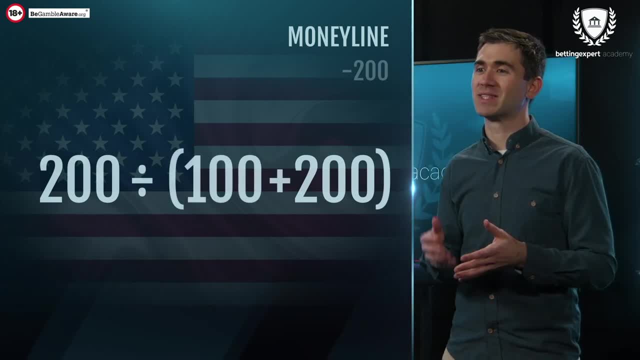 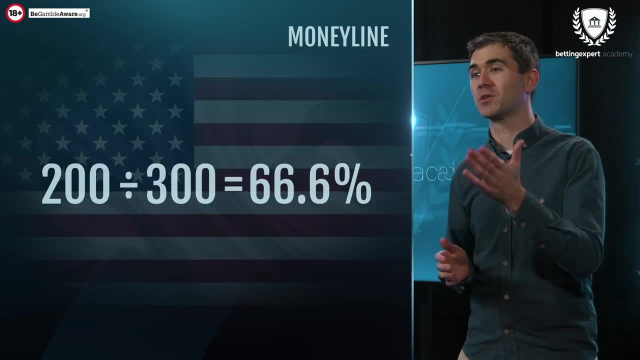 So an example might be minus 200. So here we would take 200 and divide it by 300, giving an implied probability of 66%. So here, by the way, you can also clearly see that minus American odds indicate a favorite. 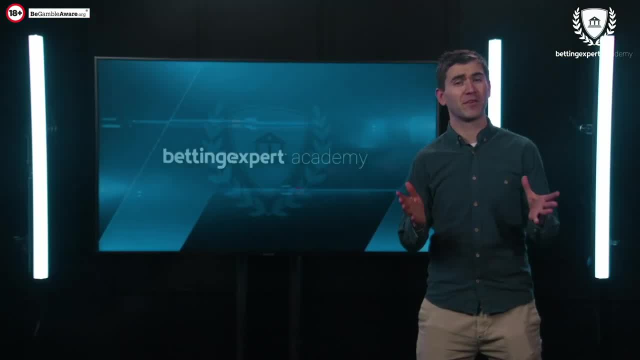 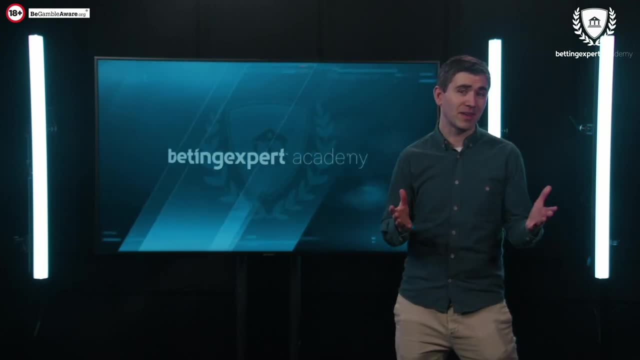 while plus American odds indicate an underdog. Now, hopefully, that all makes sense, But let's expand a bit more on why doing these calculations is important when betting. Well, it gives you a good idea of how likely a bookmaker sees an outcome actually being. You can then compare that to your own. 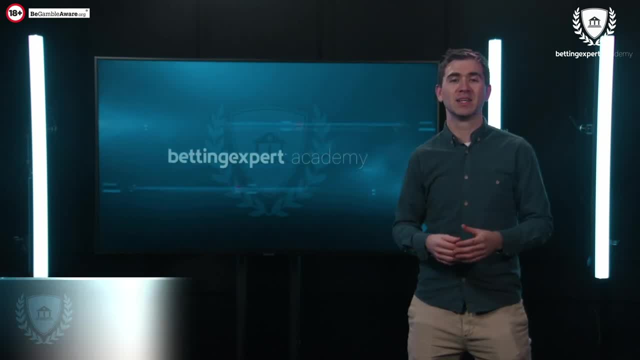 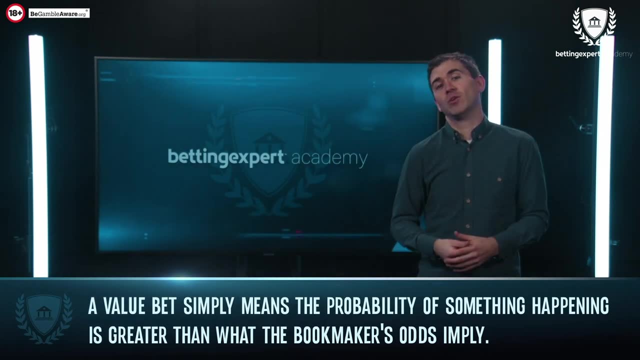 analysis and assess the results. So let's take a look at that. So let's take a look at the results. So a value bet simply means the probability of something happening is greater than what the bookmaker's odds imply, meaning you're more likely to win. So an easy example here would be if a 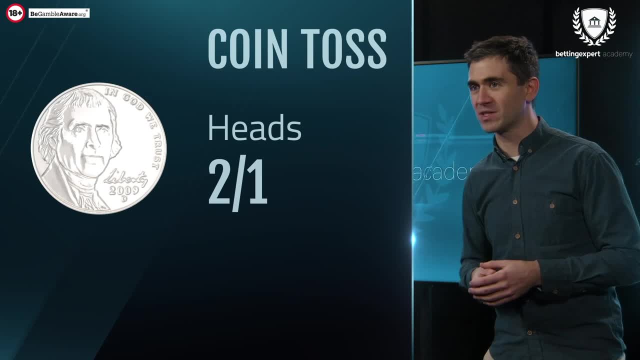 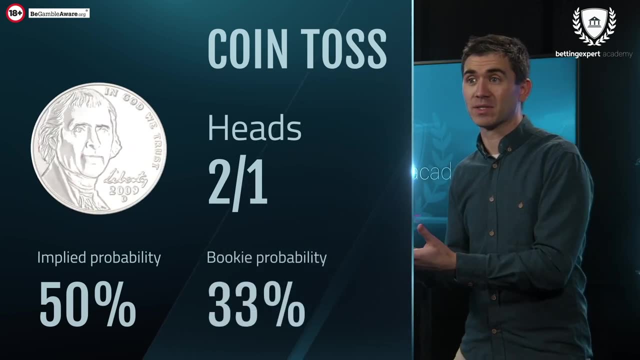 bookmaker offered you two to one for heads to be the outcome of a coin toss. Now we know the outcome is 50% likely to be heads or tails, But the bookies odds imply that it's only 33% that heads will happen. So we should be backing heads every single time Now. in practice you'll be hard pressed. 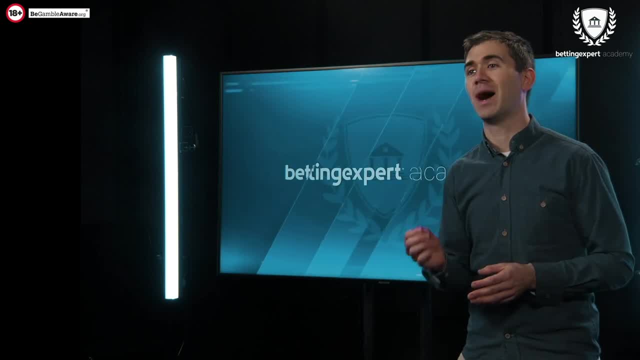 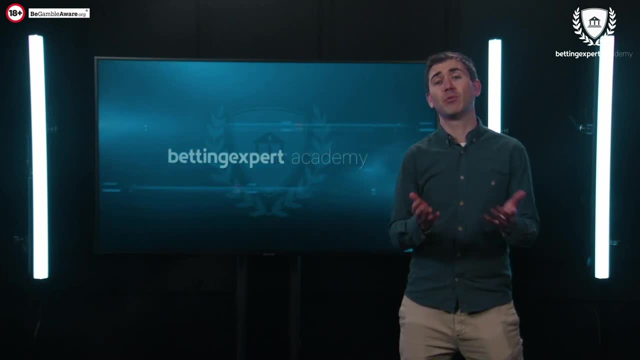 to actually find a bookmaker that generous but value bets do happen all the time. One extreme example of this is actually a recent FA Cup match between Aston Villa and Liverpool. Liverpool were initially priced around evens or 2.0 or minus 100, which is an implied probability of 50%, But illness. 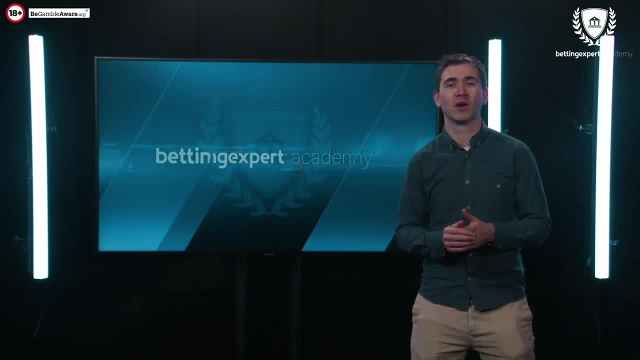 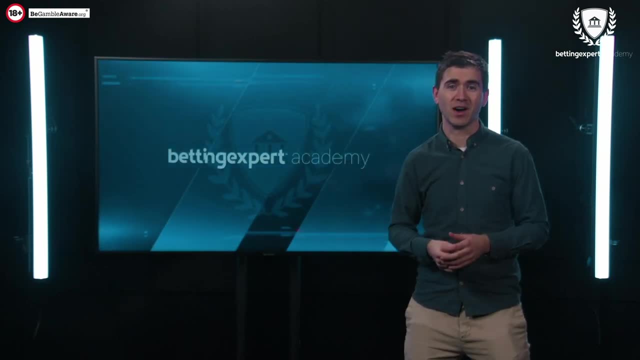 spread through the Villa squad and it became clear that Villa would only field a weakened team. So Liverpool's odds fell dramatically to give an implied probability that they would win around 90% of the time. So if you backtracked to the bookmaker's odds, you can see that the bookmaker